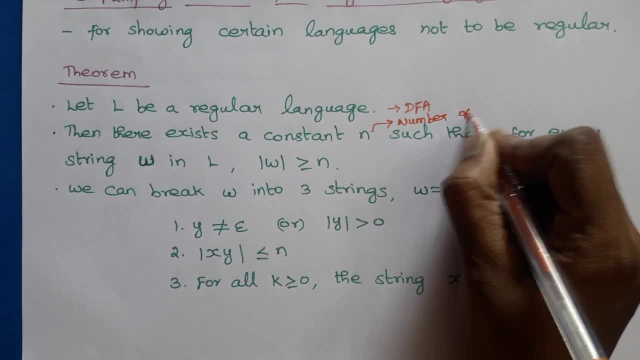 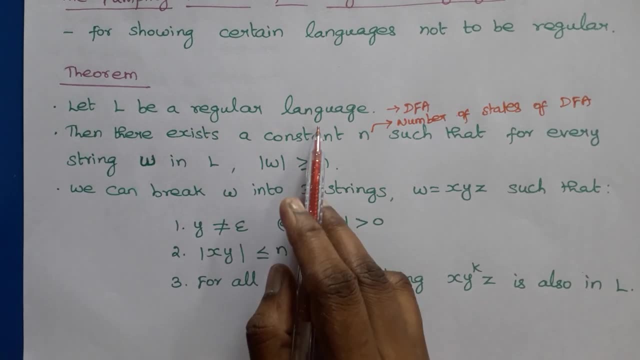 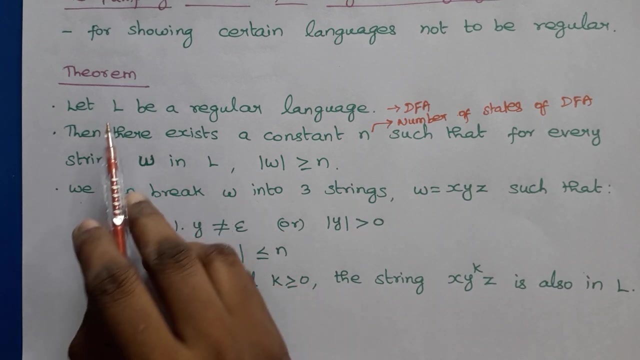 DFA: Number of states of DFA. So let L be a regular language. then there exists a constant n, such that for every string w in L, L is a language. So it consists of set of strings, right? So for that, for any string w, the length of w should be greater than or equal to n, That is. 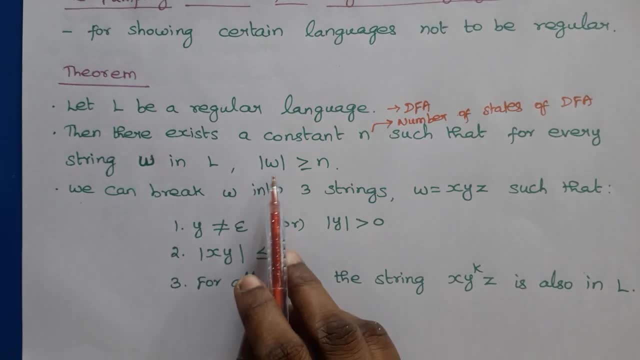 we need to choose a string from L and its length must be greater than or equal to this constant n. This is otherwise known as pumping length. So this length of w length of the string should be greater than or equal to n. So this length of w length of the string should be greater than or. 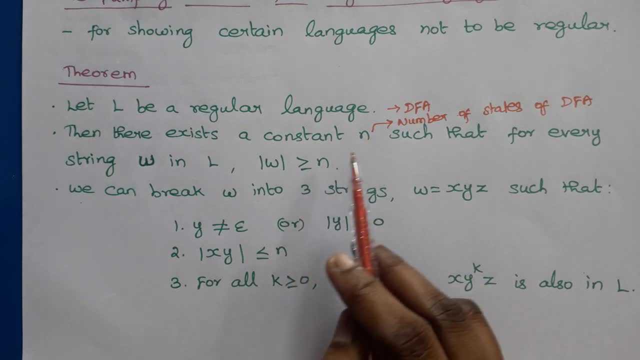 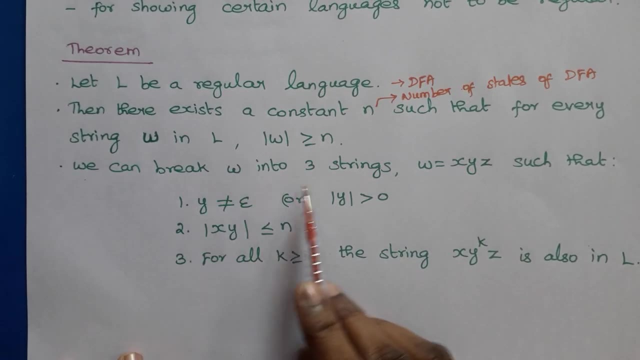 equal to n. n means constant, that is number of states of the DFA, or we can say it as pumping length. So now we can break w into three strings. That is, w is equal to x, y and z. These are the substrings of w. So we can split w into x, y, z with three conditions Here. the middle string, y, 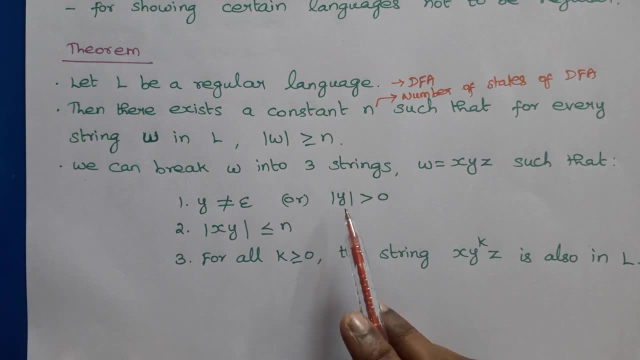 not equal to epsilon. That is, the length of y is not equal to epsilon. So we can break w into: y should be greater than zero. y should be at least one length. Okay, it is a non-empty string. and another condition is the length of x. y is less than or equal to n. That is together. 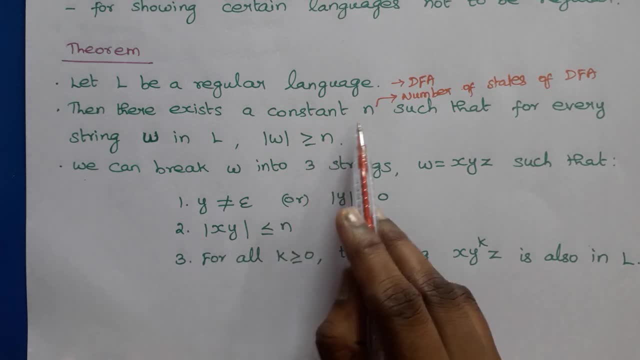 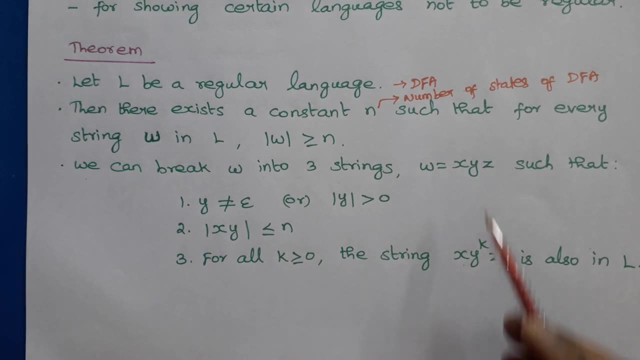 the length of x, y together is less than or equal to this constant n and for all k greater than or equal to zero. the string x y to the power, k z is also in n, And that is if we power k? y to the power. 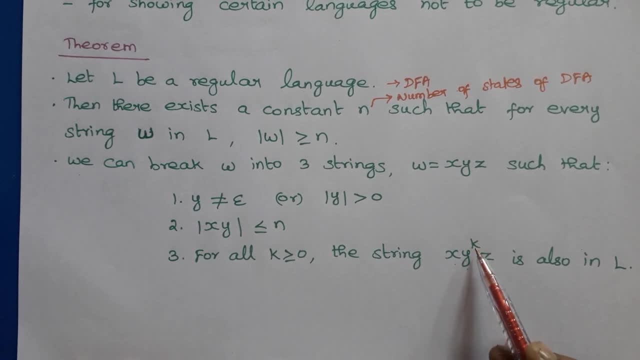 k. we can pump the non-empty string y k number of times, that is including zero. We can pump this y any number of times including zero. That is, we can remove y or y can be repeated. increased any number of times means the resulting string must also be in l. Then only we can say that the language is. 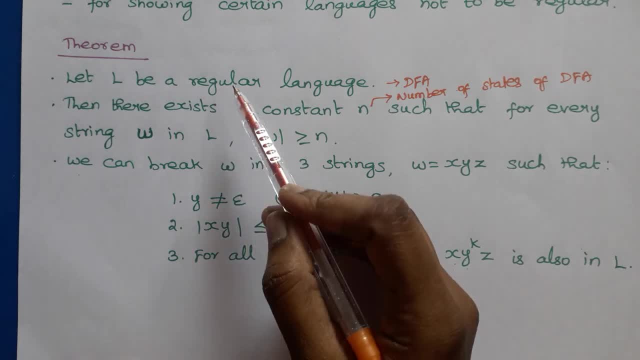 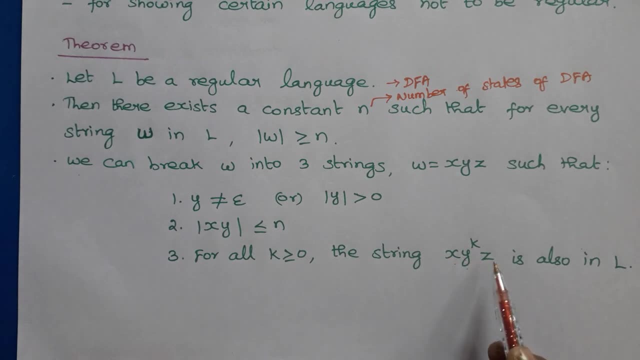 regular. So to prove a language is not regular, we have to start considering l be a regular language. At the end here, x, y to the power, k, z, we will get the contradiction result, That is, it is not belonging to l. So in that case we can say that the given language is not a regular language. 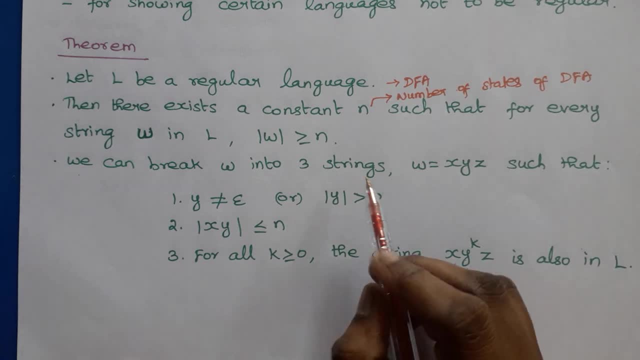 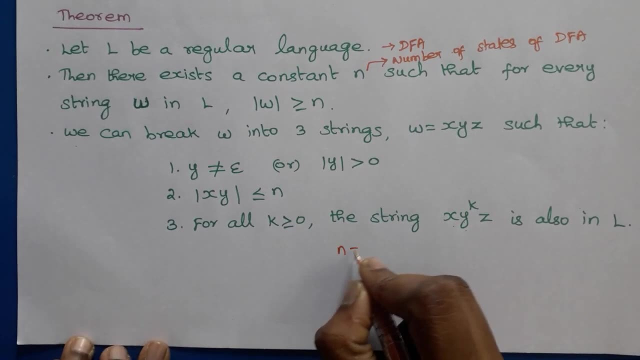 So here how x, y to the power, k, z, is considered. If we consider w, length of w is greater than or equal to n. So assume that n is 3.. So what is the meaning of this? w has some three symbols. 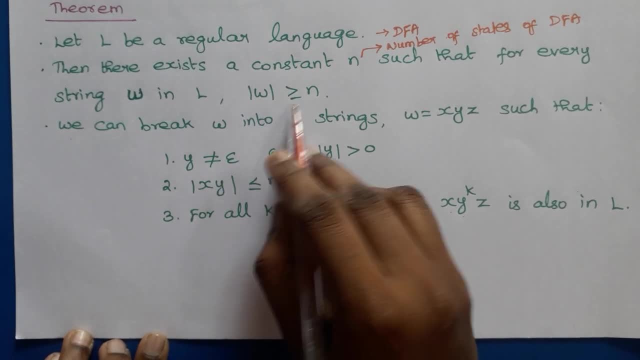 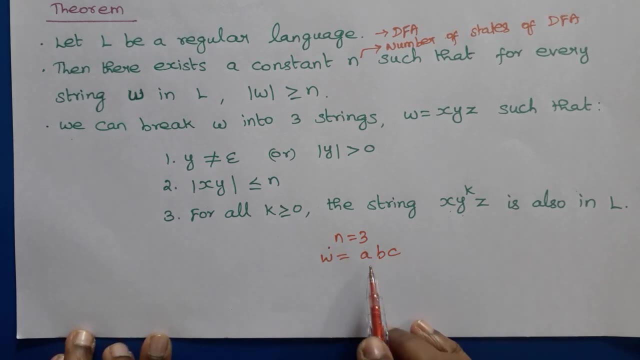 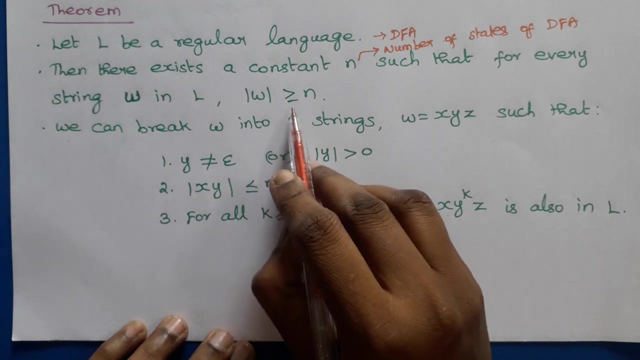 The length of w. length of w is greater than or equal to n, So we have considered n equal to 3.. That is, we are considering the same number of n number of symbols. W has n number of symbols, but it can also have 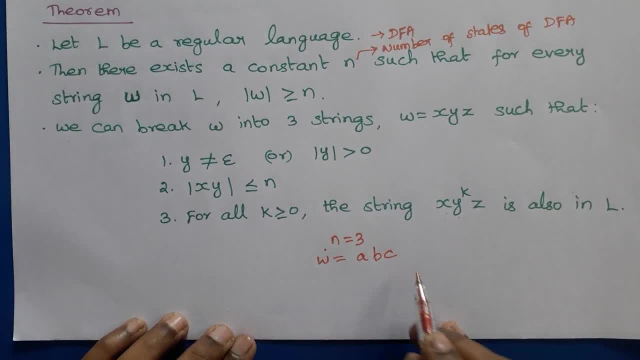 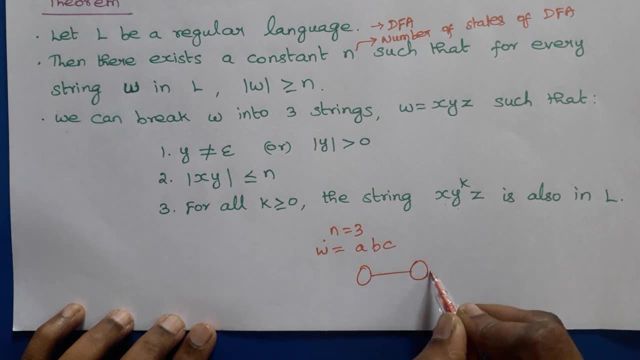 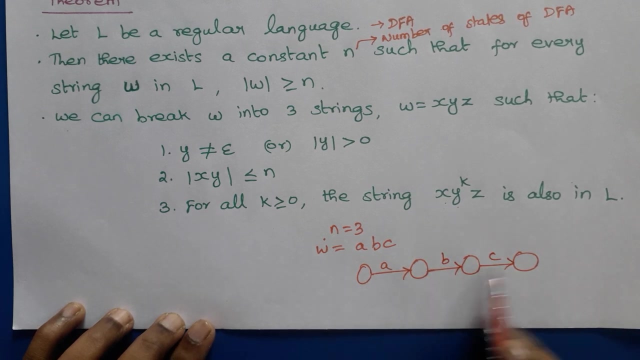 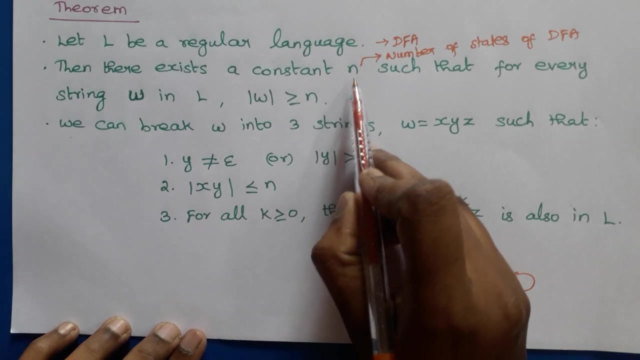 greater than n. Suppose, if w has n number of symbols, how many states we need to construct DFA? We need four distincts Distinct states. right, Distinct states means we need four. For taking three symbols, we need four distinct states, But here the condition is n. It can have n number of states. The DFA will have n. 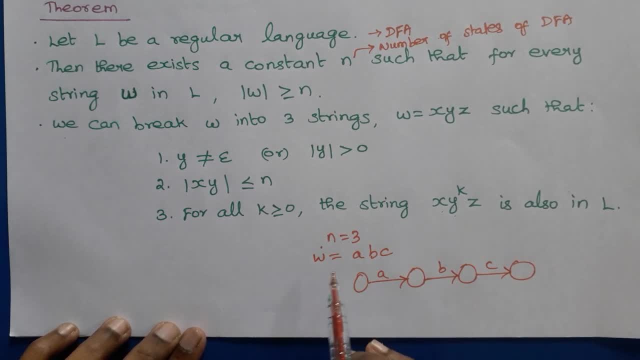 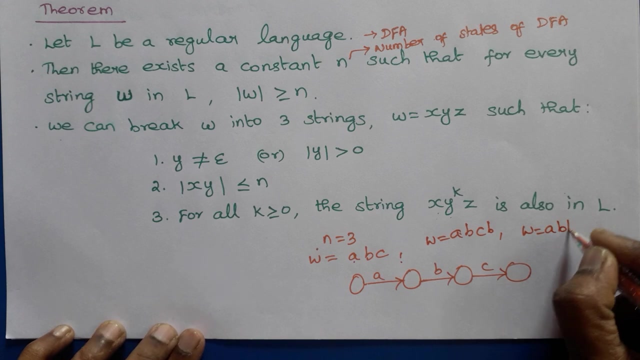 number of states. So n means 3.. So that at least a cycle will occur, right, Because this is a minimum condition, W is 3.. But it may also be a, b, c, b a, b, b, b, a, like that. So we cannot have n plus one number of states, right Actually? 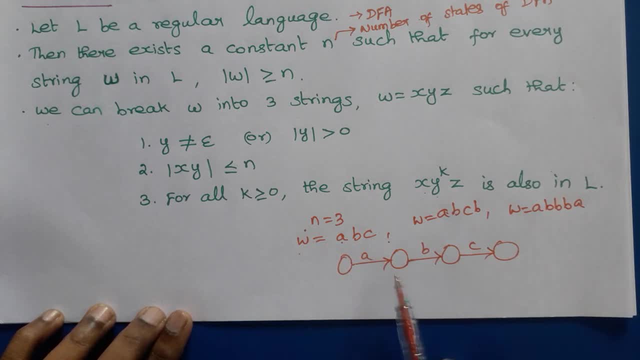 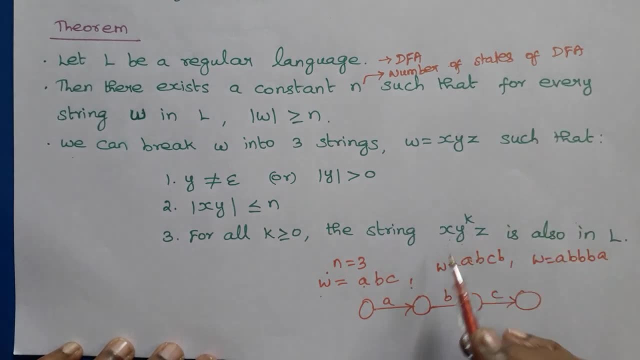 if w has n symbols, then we need n plus one number of states. But it is not possible because here the condition is it can have n number of states. So it should be pumped Some symbols. some symbols will go to the same states as the previous symbols. So here we are considering middle. 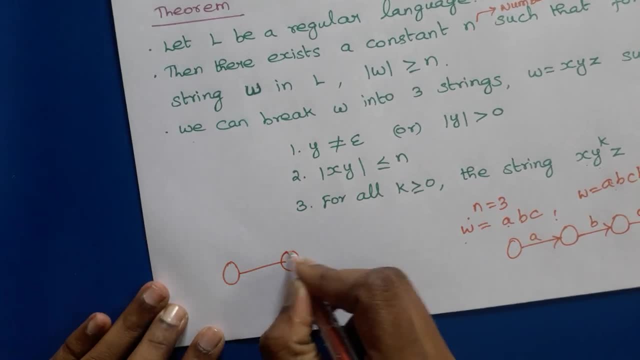 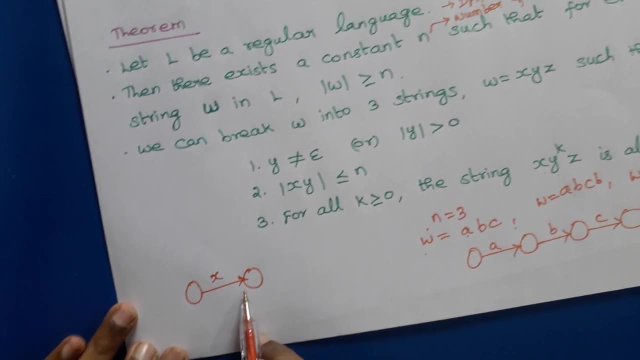 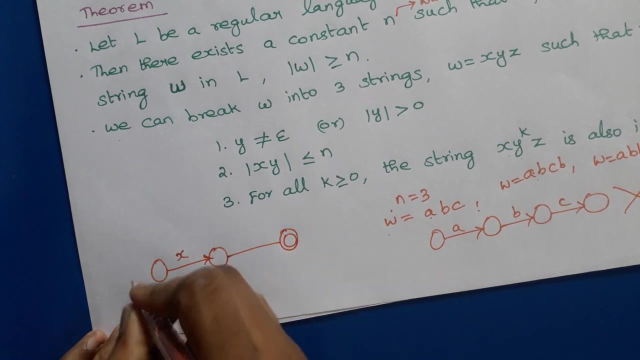 middle symbol is pumped So that x. this is not possible. So for x: from the start state it can go to another state, Because in this example we have only three states, And this is the start state and this one is final state. So for x and z are here compulsory, y can. 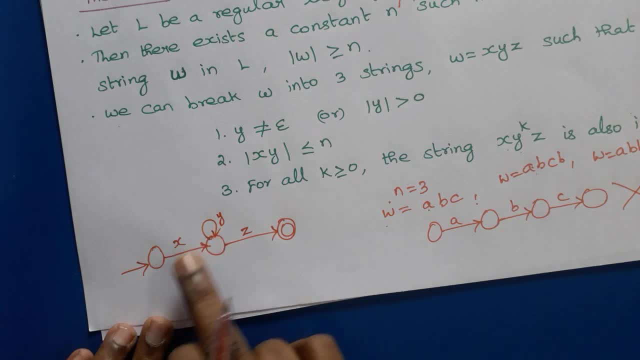 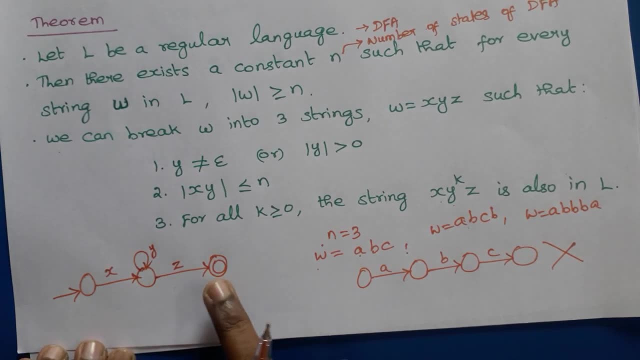 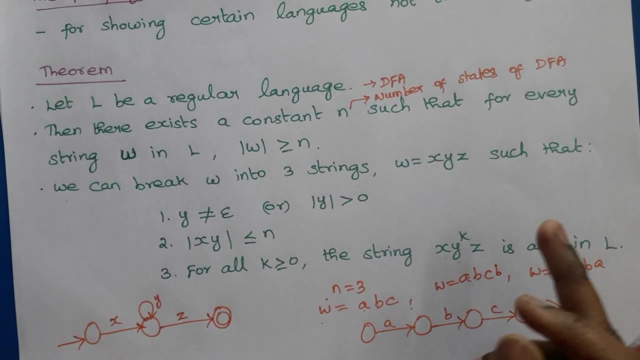 be pumped any number of times, So it may be zero also. So x, any number of y- can be pumped. y followed by z means the resulting string should also be in l. the meaning is it should reach the final state, so that if we prove this then the language is regular. but we will get contradiction. 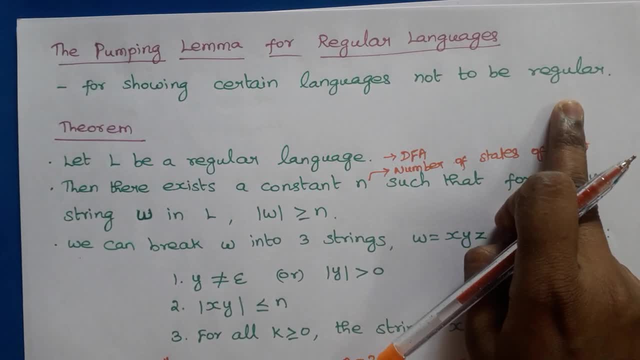 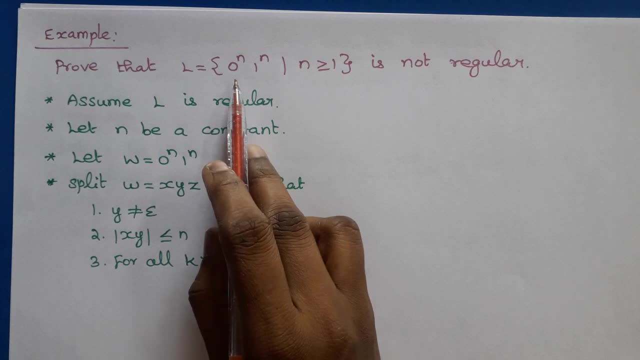 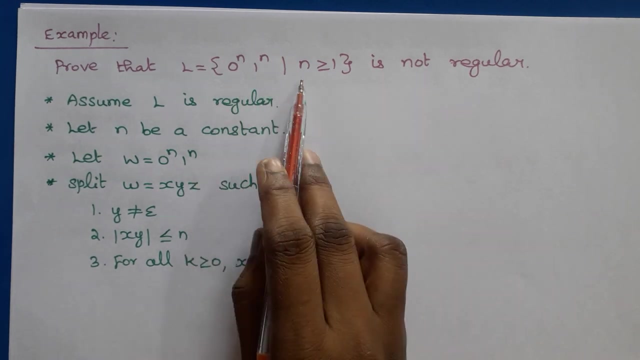 here because pumping lemma is used for proving the language is not regular. now we will see an example. so consider this example: prove that l is equal to 0 to the power n, 1 to the power n, such that n is greater than or equal to 1, is not regular. actually, this language is not regular, right. 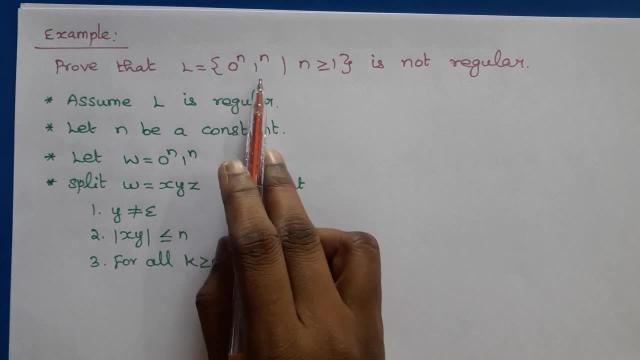 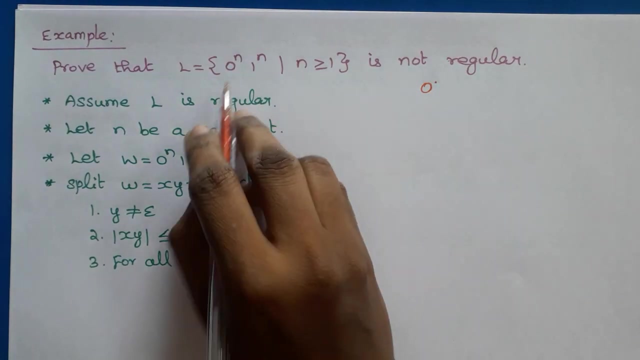 because we cannot construct dfa for this language, because here the meaning is l should accept all strings which have equal number of zeros followed by equal number of ones. here n is greater than or equal to 1, so if you substitute n as 1, we will get 1, 0, 1, 1, then 0, 0's, 1, 1's. 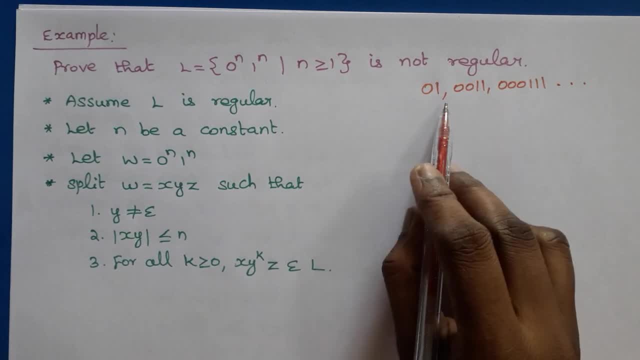 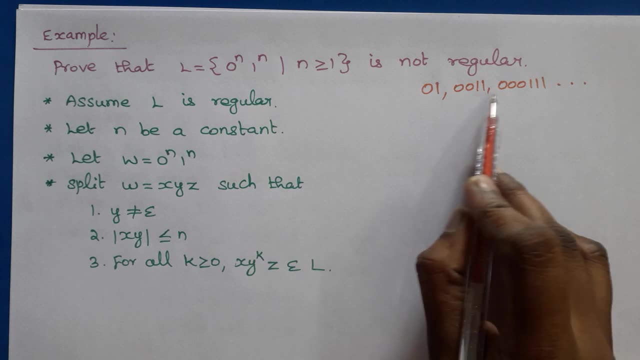 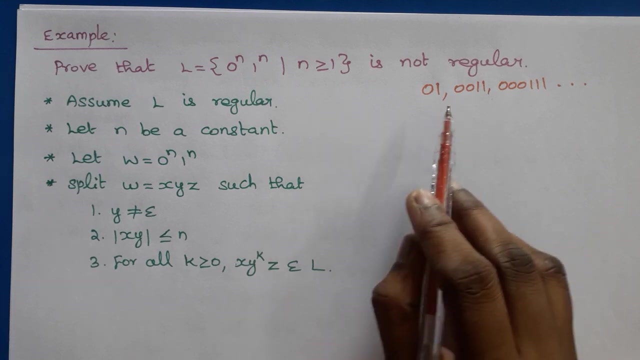 triple 0, triple 1, etc. so it should accept some number of zeros, followed by all the strings which are having zeros, followed by equal number of ones. the number of zeros and ones must be equal. but the finite automata will have only the finite automata has only the limited memory that. 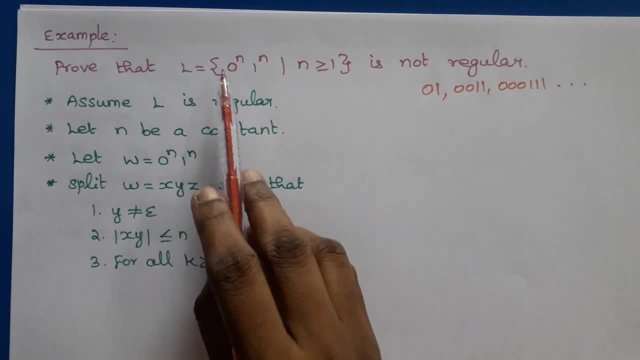 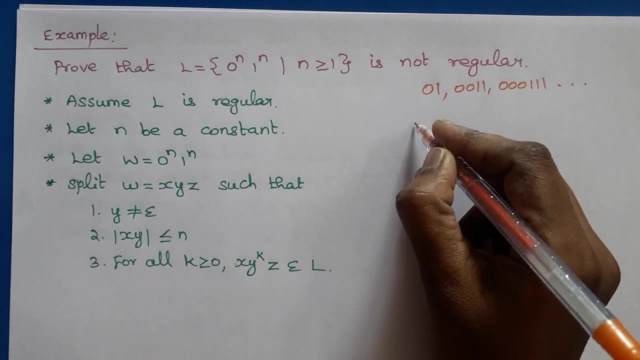 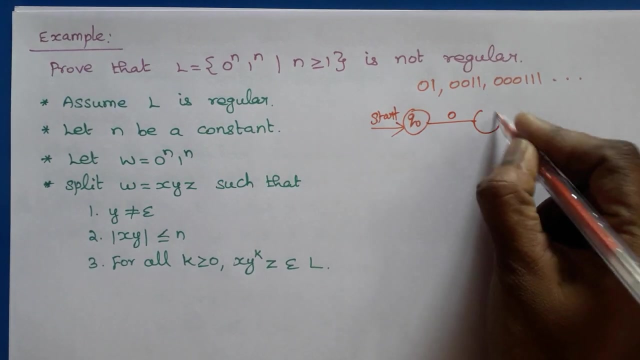 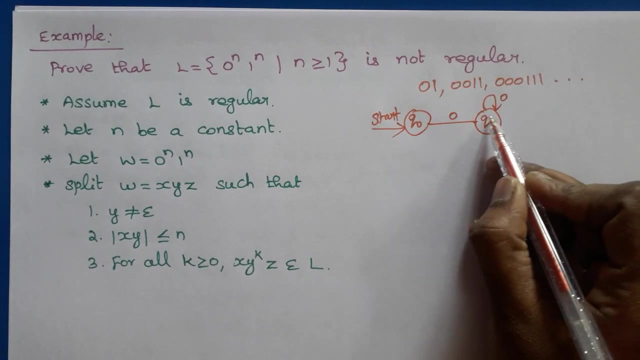 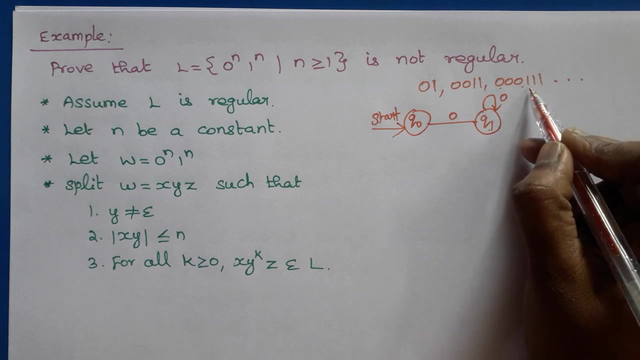 is, it has the finite memory. it cannot remember whether it has read n number of zeros or m number of zeros. if you start constructing, if dfa 1, 0 followed by number of zeros, so here, for example, consider the string 3 zeros, 1, 0, 2, 3, for after reading all the 3 zeros, it will be in state q1. now it starts reading 1. 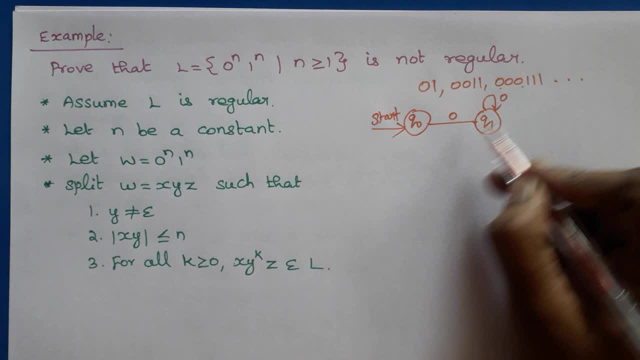 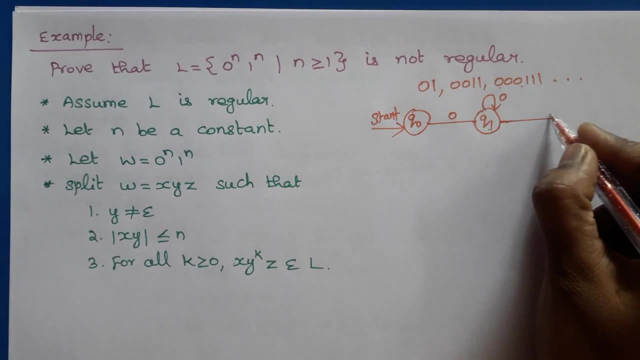 but it cannot remember whether it has read 3 zeros or 4 zeros or 5 zeros. so it cannot remember whether it has read 3 zeros or 4 zeros or 5 zeros. so it cannot match the number of zeros and ones. so if you start constructing a dfa like this, 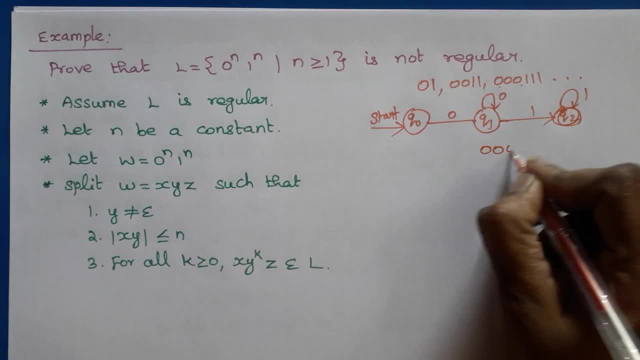 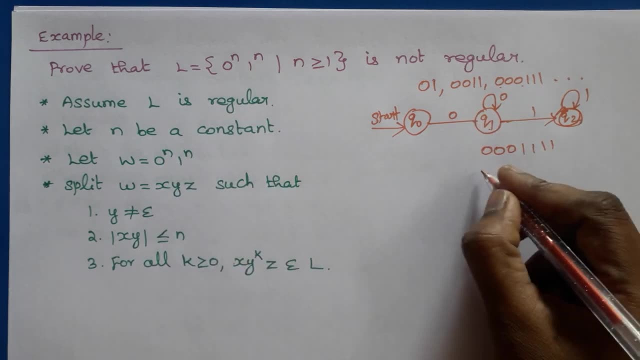 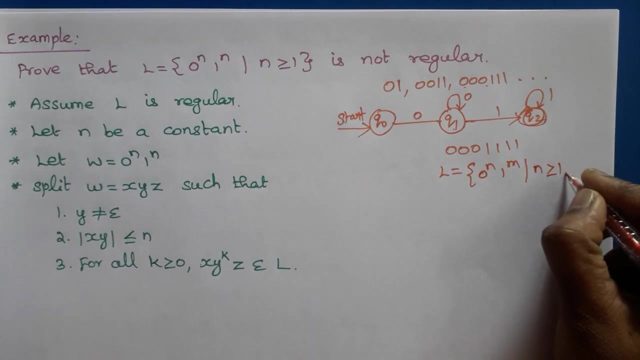 it can accept any number of zeros followed by any number of ones. so it is not the dfa for this language. so suppose if the language is 0 to the power n, 1 to the power m, such that n is greater than or equal to 1 and m is greater than or equal to 1 means it can accept any number of zeros, or 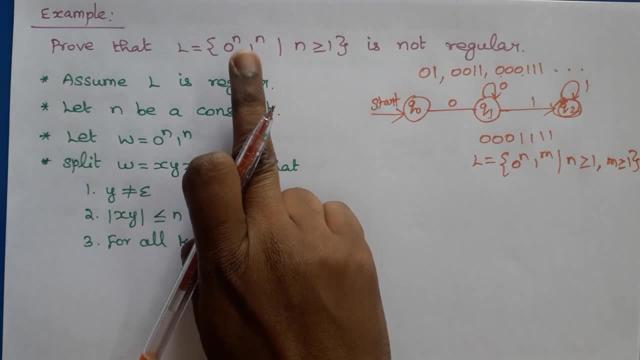 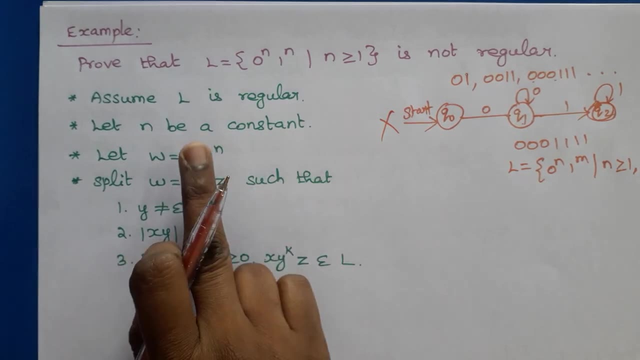 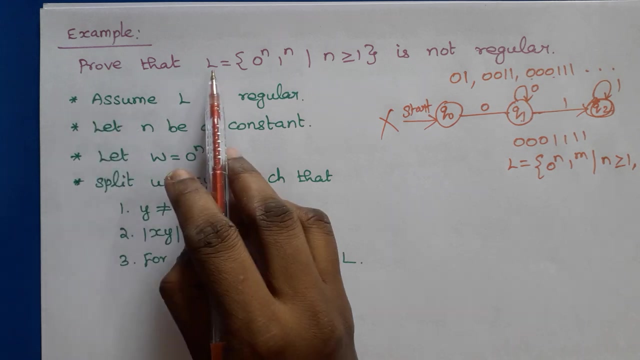 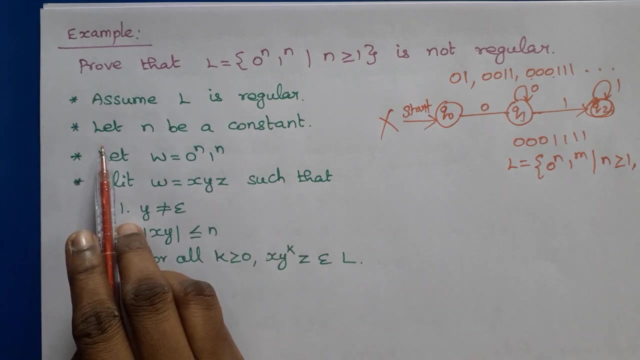 a 0. so we will go ahead and apply this formula and that output would have been equal to n. the following response is n- dfa, and i compared this number of zeros with thealled zeros and actually 0 didn't accept it. so for 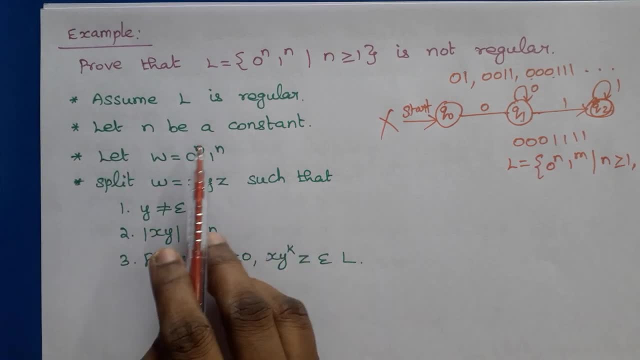 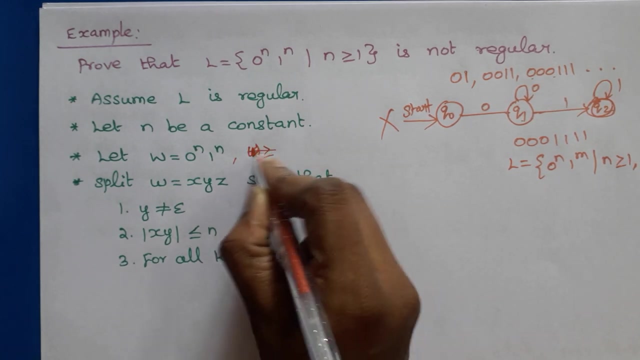 example. let me try using the equation again that says: here: nothing but 0 is equal to 0. that is it. we can write it as n be a constant. then we need to choose a string, w, and the condition is: the length of w should be greater than or equal to n. length of w should be greater than or equal to. 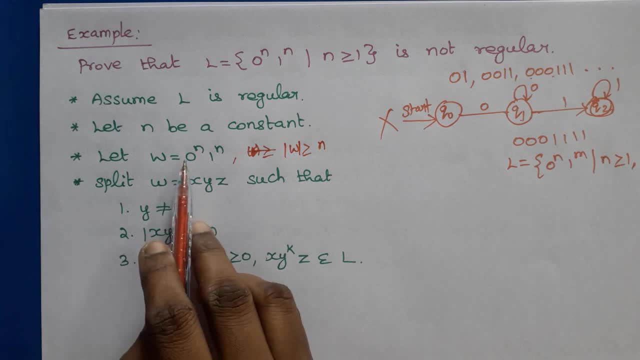 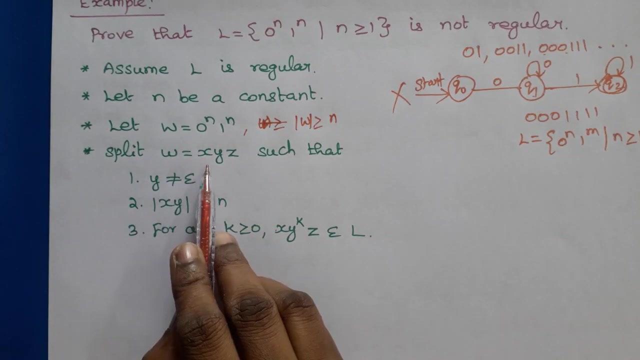 n. so here we have chosen 0 to the power n, 1 to the power n as a string, w, because here the length is greater than. a length of w is greater than n. the length is 2n, right, so length of w is greater than or equal to n. here then we need to split w in the form of three strings: x, y, z. with the three 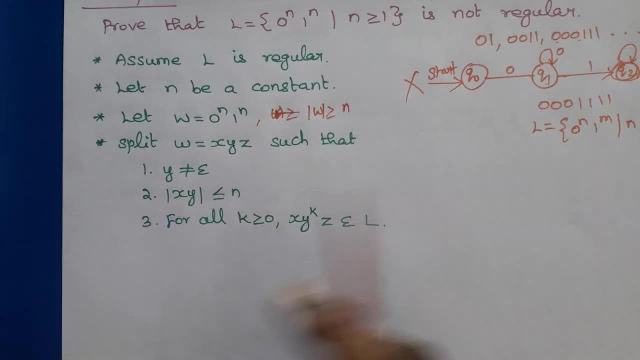 conditions. this we have already discussed in the last in the definition. so now we have to consider the string w is equal to 0 to the power n, 1 to the power n right, and assume that n equals 2.. If n equals 2, then what about w? w is 0, 0, 1, 1, then we need to split this w into x, y, z and here: 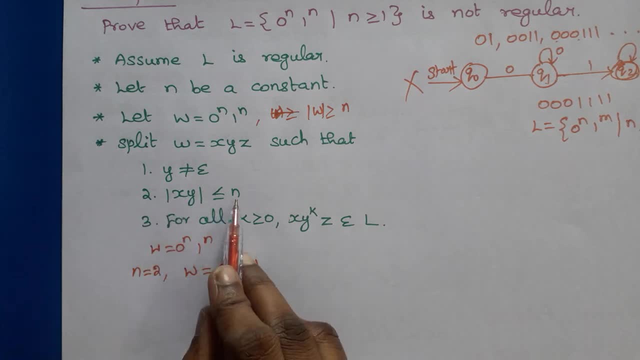 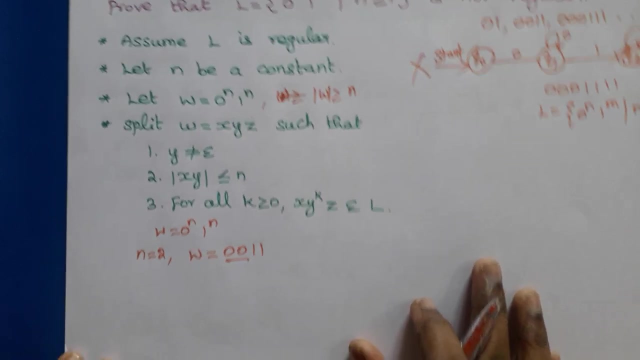 the second condition is length of x? y is less than or equal to n. that is, length of x? y is at least at most n, so it can have maximum of n number of symbols, so that x? y can be 0, 0 right, because 0 is greater than or equal to n. so we need to split this w into x, y, z. and here the second. 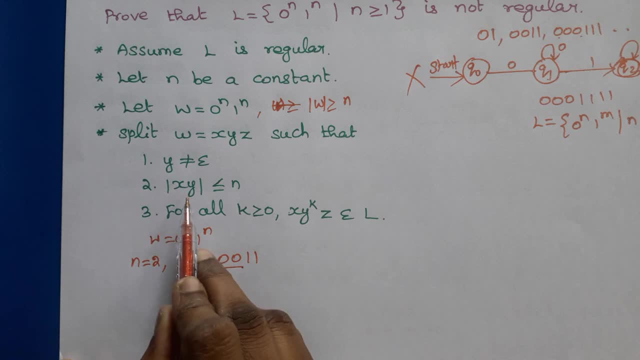 condition is: length of x? y is 0 to the power n, 1 to the power n and the length of x? y is less than or equal to n means x? y contains all zeros in the string, so that x? y is equal to 0, 0 and then. 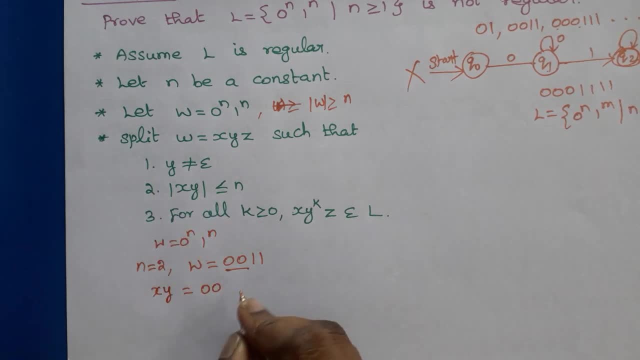 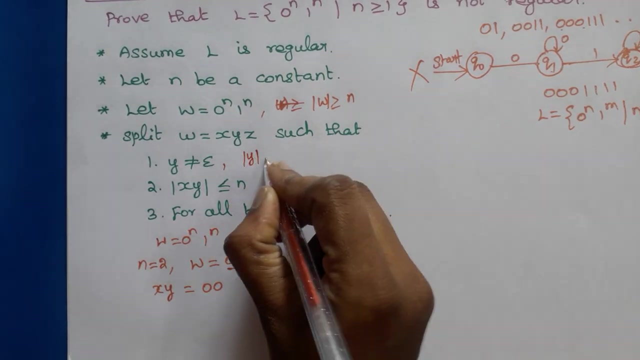 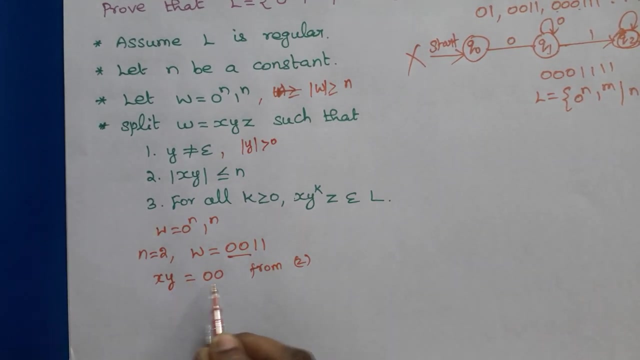 so this is from rule number 2. from 2, we have written this and, as per rule 1, y is not equal to epsilon right, or we can say it as a 0, so length of y is greater than 0. so at least y has one symbol. so from this x, y is equal to 0, 0. 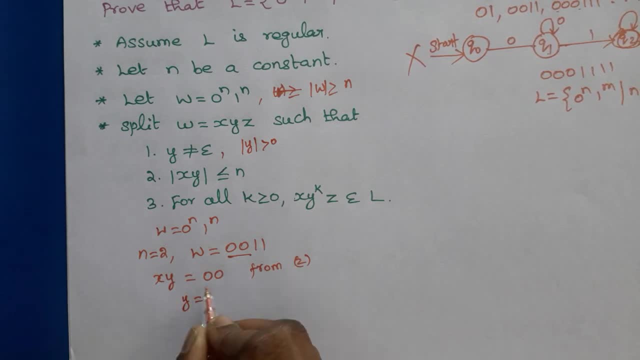 we can consider: y equals 0, so y is 0. means what about x? the remaining 0? so x equals 0, y equals 0. then what about z? the remaining symbols of the? w is z, so z is 1, 1. okay, so from rule 2. 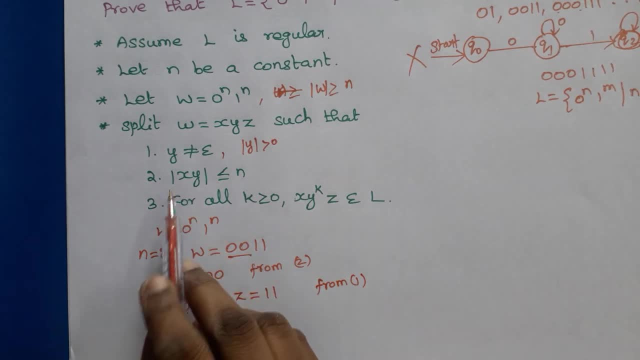 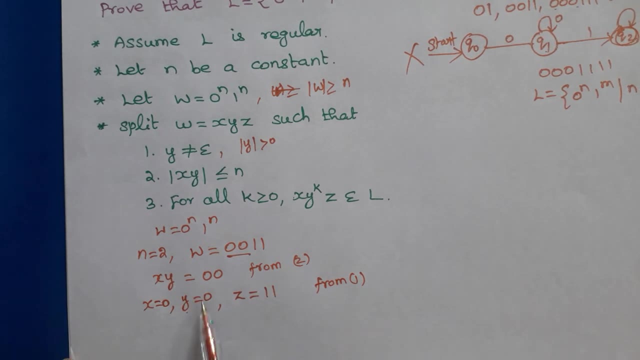 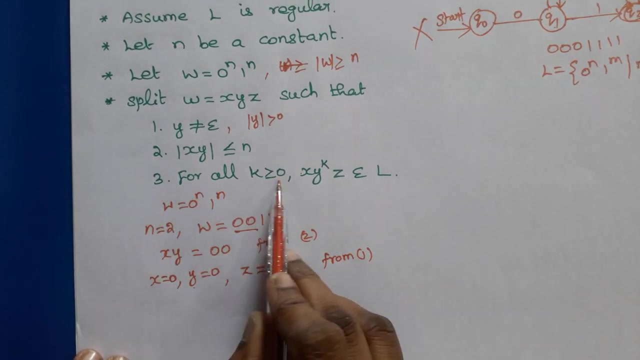 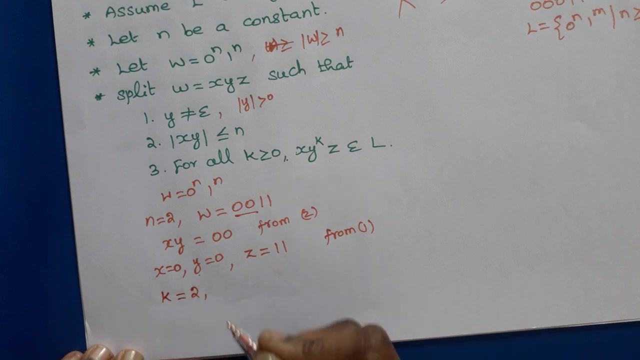 as per rule 2, length of x, y is double zeros and from rule 1 we have written y as 0 and x is 0. z is remaining symbols. now we have to prove the third condition, that is, for all k greater than or equal to 0, x, y to the power k, z belongs to l, so assume that k equals 2. so if you consider k, 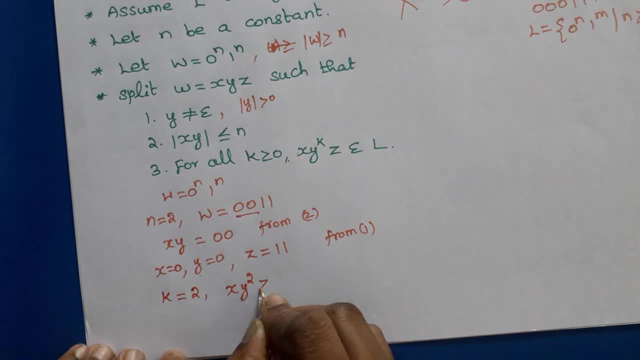 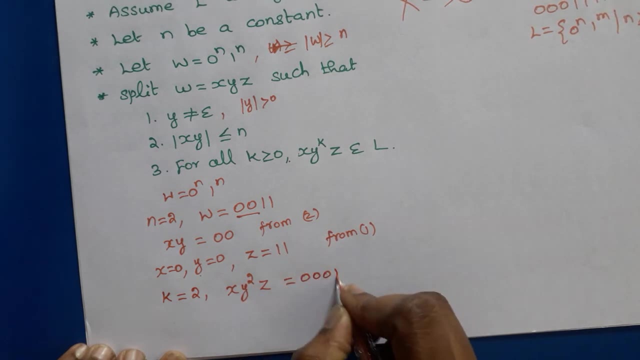 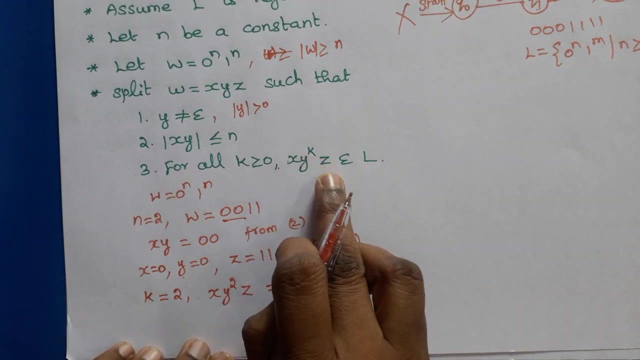 equals to x, y to the power. 2. z equals x means 0, y is 0, so y square means 0, 0, then 1, 1. so here we have got the string triple 0, double 1. actually, the condition is x, y to the power k. z belongs to l, so l means